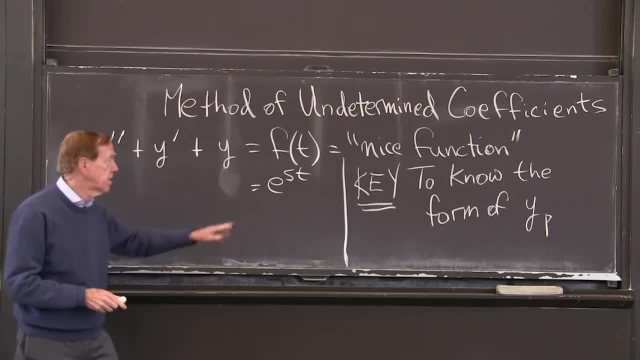 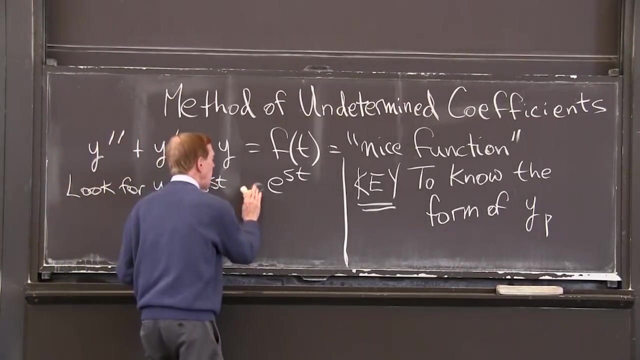 in the equation. Now do you remember what we look for? when the right-hand side is e to the st, Then look for: y equals some constant times: e to the st Right When f of t. maybe I'll put the equal sign down there. 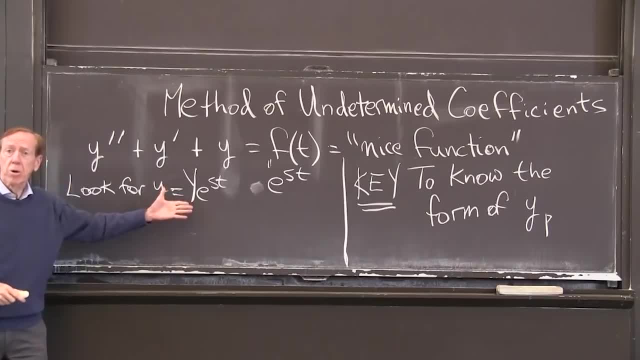 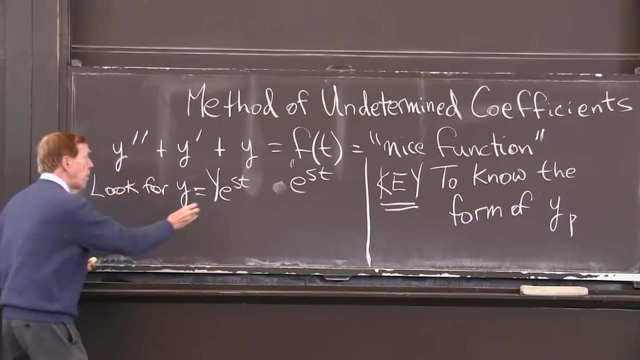 If f of t is e to the st, then I just look for a multiple of it. That's the set. That's one coefficient To be determined by. substitute this into the equation. Do you remember the results? So this is our best example. 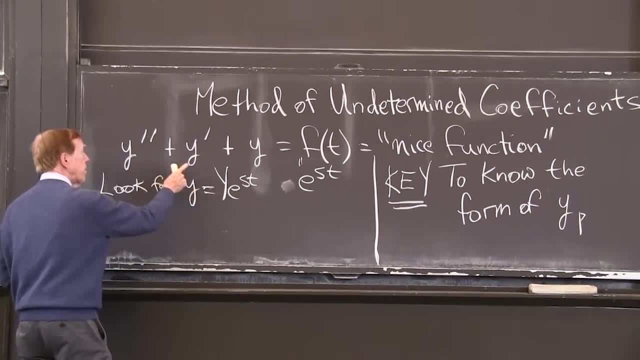 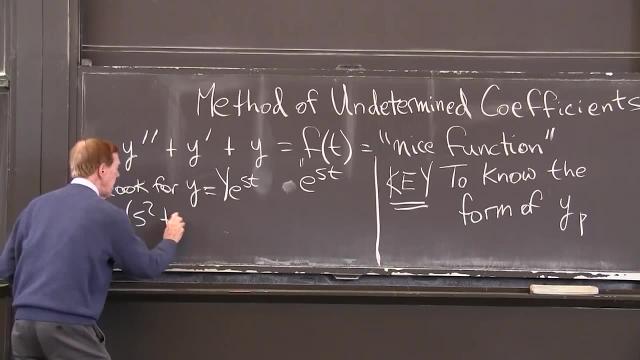 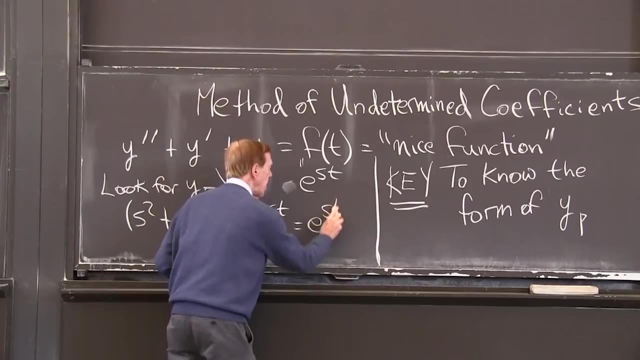 When I put this in the equation, I'll get: the derivative brings an s. Second derivative brings another s. So I get s squared and an s and a 1 times y e to the st is equal to e to the st. We've done that before. 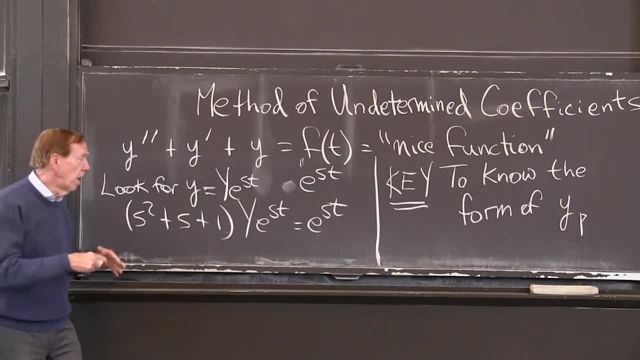 Here we see it as a case with undetermined coefficient y, But by plugging it in I've discovered that y is 1 over that. So that's a nice function. then e to the st is a nice function. What are the other nice functions? 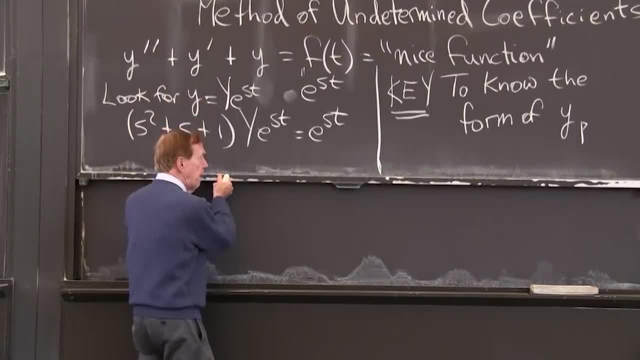 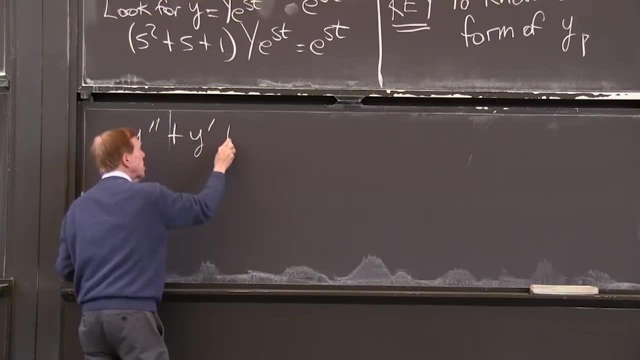 So now let me move to the other board, next board, and ask: what other right-hand sides could we solve? So I'll say: Keep this left-hand side equal to. So e to the st was 1.. What about t? What about t? 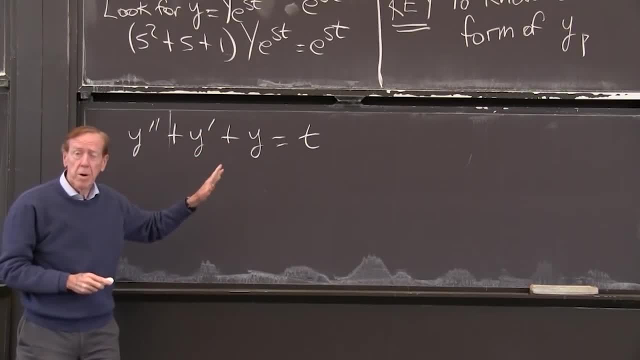 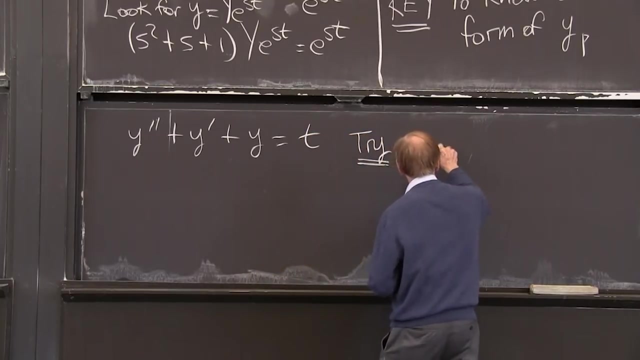 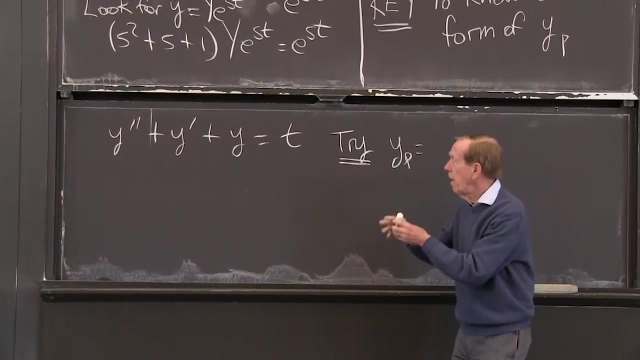 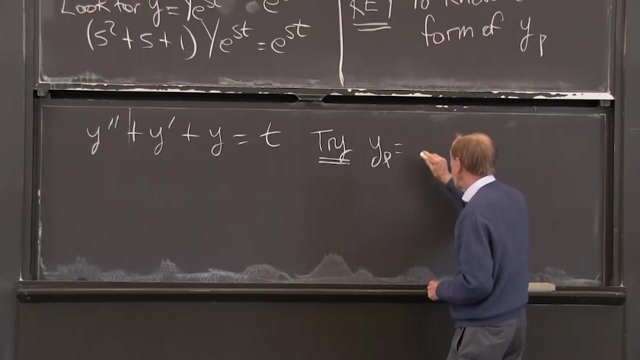 A polynomial Well that only has one term. So what would be a particular solution to that equation? So I really have to say what is the trie y particular equals. Now, if I see a t there, then I'm going to look for a t in y and I'll also look for a constant. 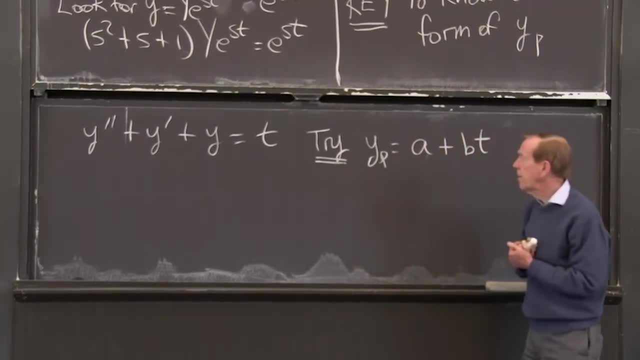 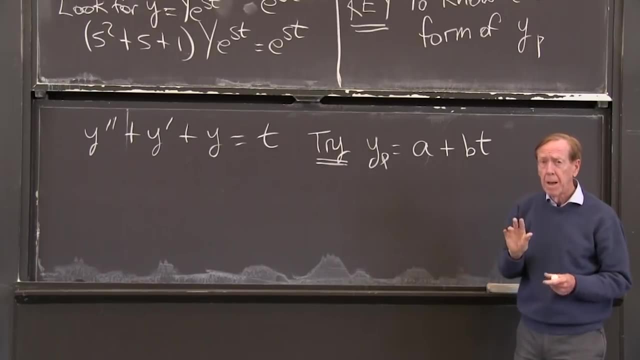 So a plus bt would be the correct form to look for. Let me just show you how that works. So this now has two undetermined coefficients and we determine them By putting that into the equation and making it right. So trie yp is a plus bt in this equation. 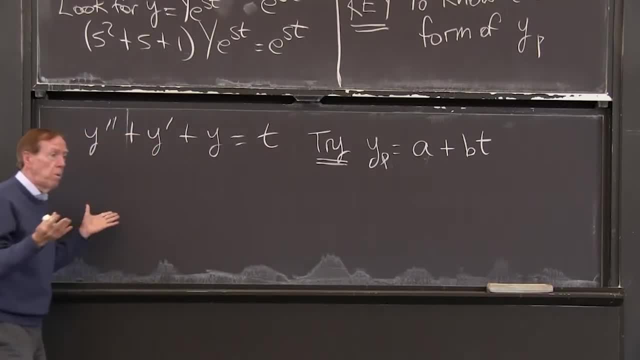 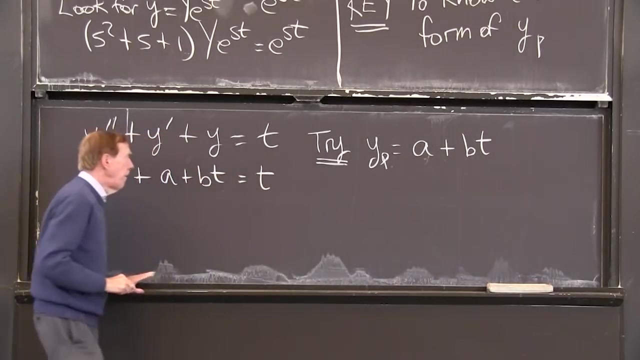 OK, the second derivative of a plus bt is 0. The first derivative of that is b. So I get a b from that And y itself is a plus bt And that's supposed to give t. You see, I plugged it in. 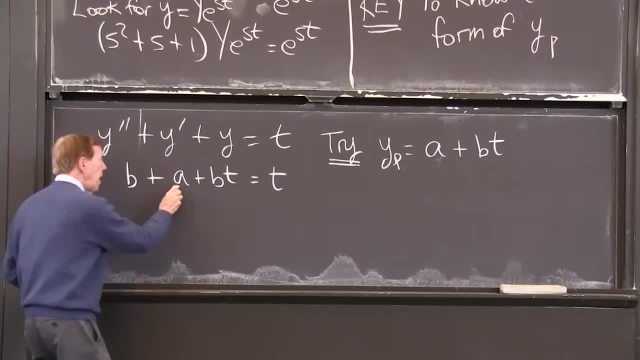 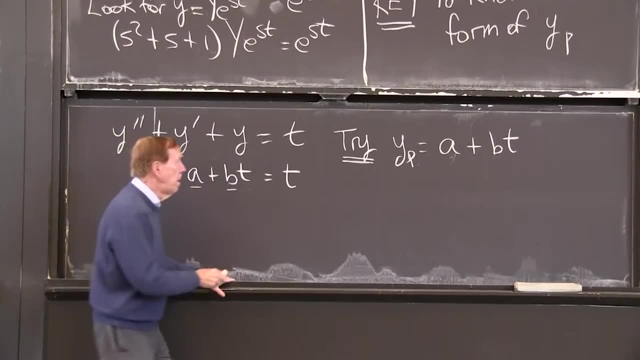 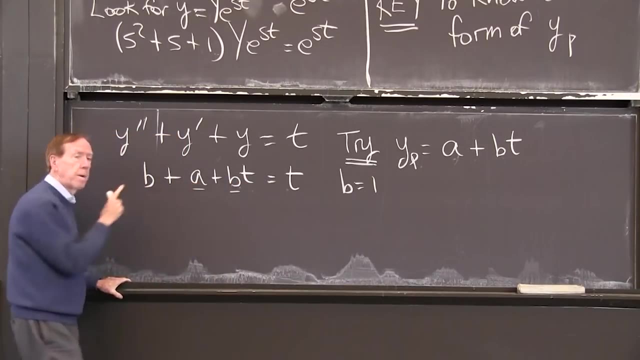 I got to this equation. Now I can determine a and b by matching t, So that b has to be 1.. We get b equal to 1. So that t equals t. But if b is 1, I need a to be minus 1 to cancel that. 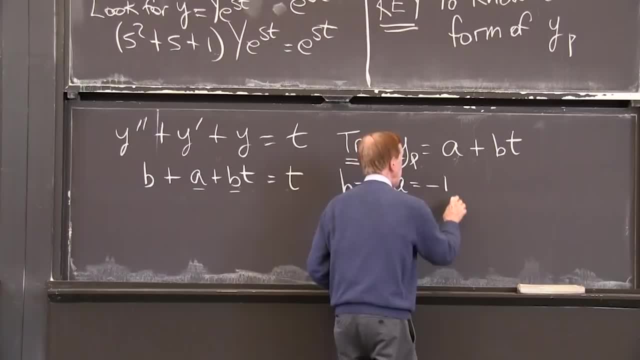 So a is minus 1.. And my answer is minus 1.. So a is minus 1.. And my answer is minus 1.. And my answer is minus 1.. Minus 1 plus 1t t, minus 1.. 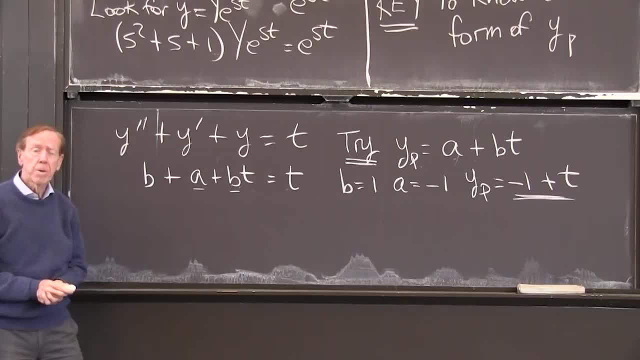 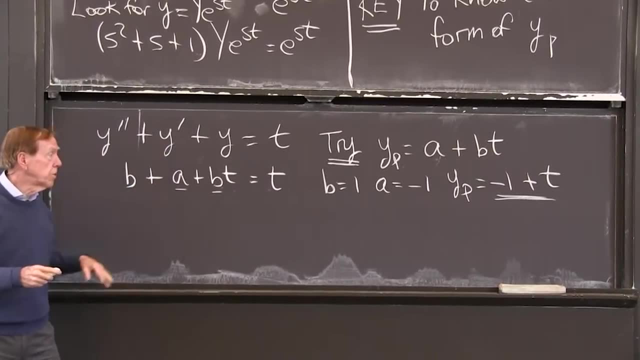 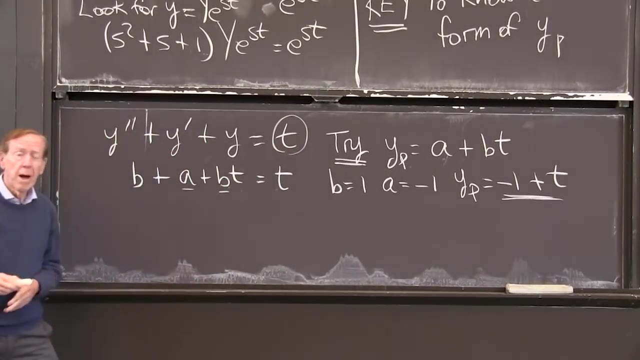 And if I put that into the equation it'll be correct. So I have found a particular solution, And that's my goal, because I know how to find null solutions And then together that's the complete solution. So we've learned what to try with polynomials. 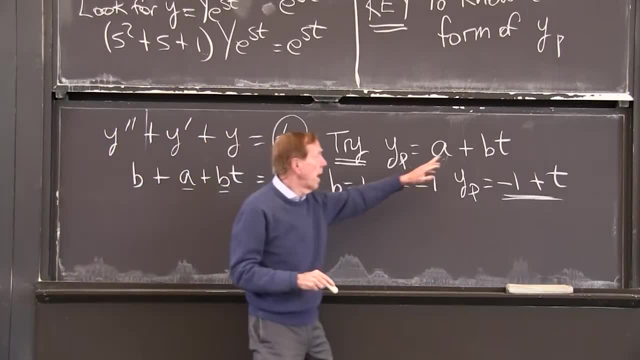 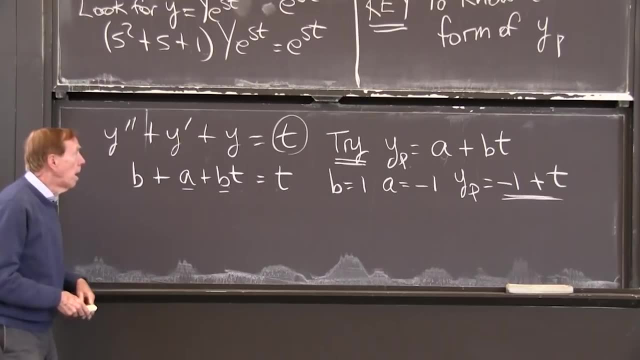 With a power of t, we want to include that power and all lower powers all the way down through the constants. OK With exponentials, we just have to include the exponential. What next? How about sine t or cosine t, Say sine t. 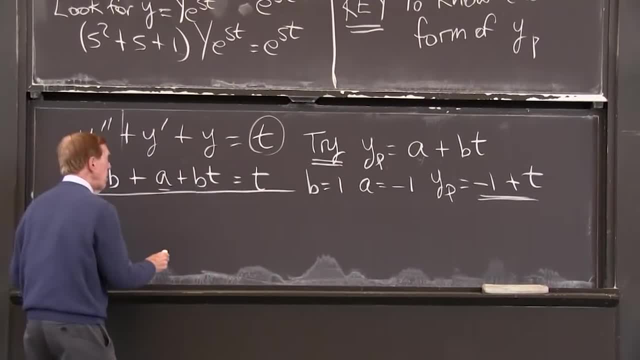 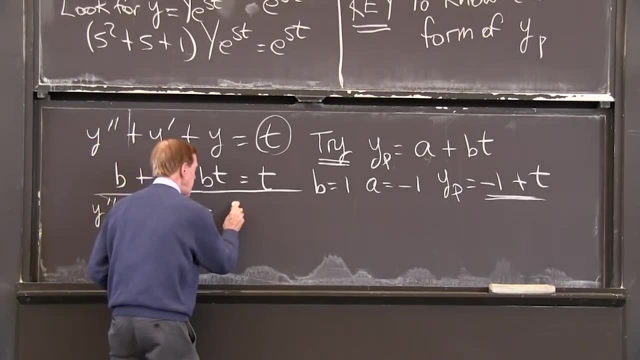 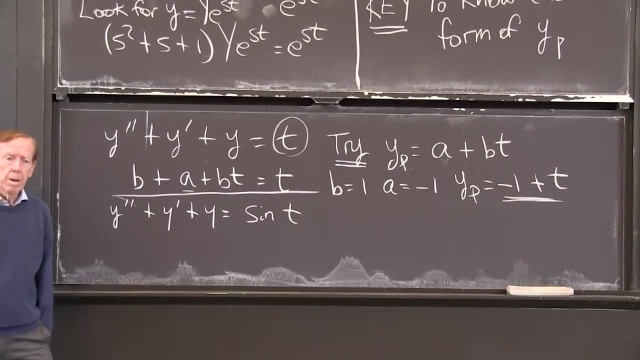 All right, So that case works. Now we want to try y double prime plus y. prime plus y equals say sine t. OK, What form do we assume for that? Well, I can tell you quickly: we assume a sine t in it. 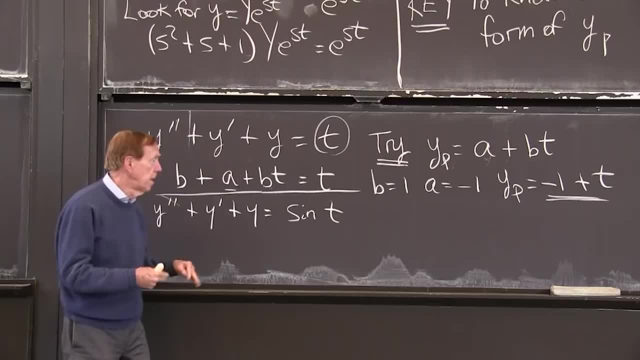 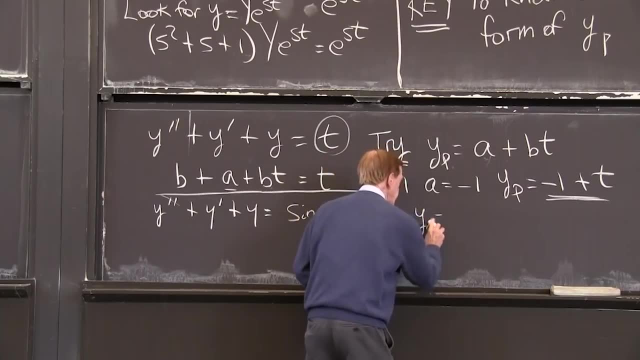 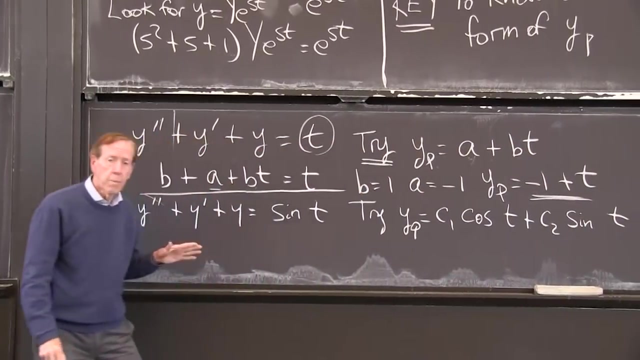 And we also need to assume a cosine t. The rule is that the things we try- so I'll try y y particular- is what we're always finding: Some c1, cos t And some c2.. Sine of t That will do it. 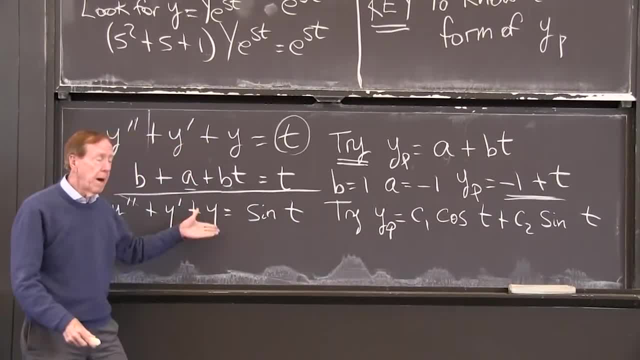 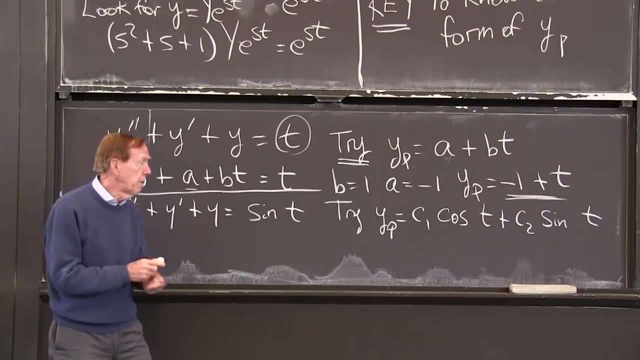 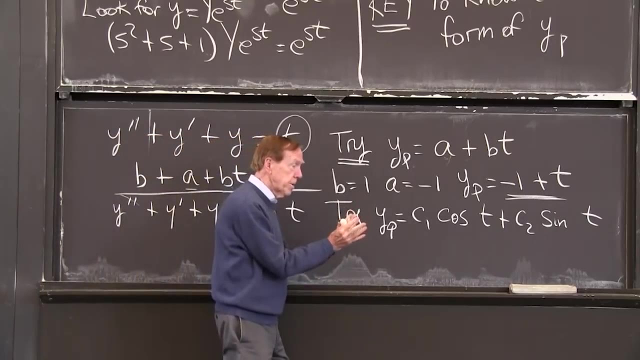 In fact, if I plug that in, I match the two sides. I determine c1 and c2.. I'm golden. Let me just comment on that. rather than doing out every step Again, the steps are: just substitute that in and make. 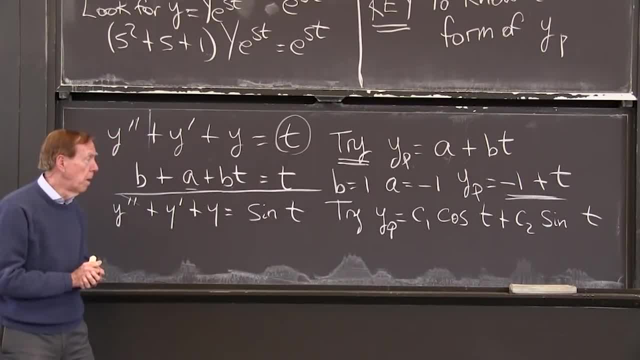 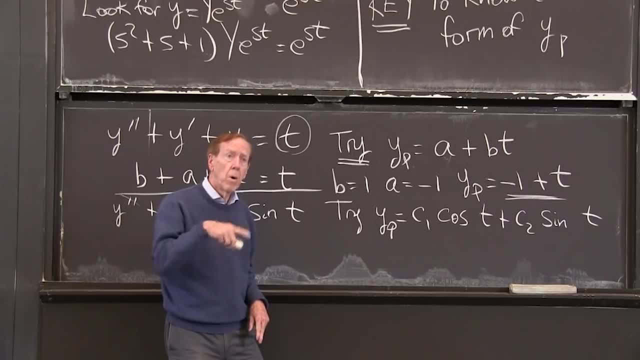 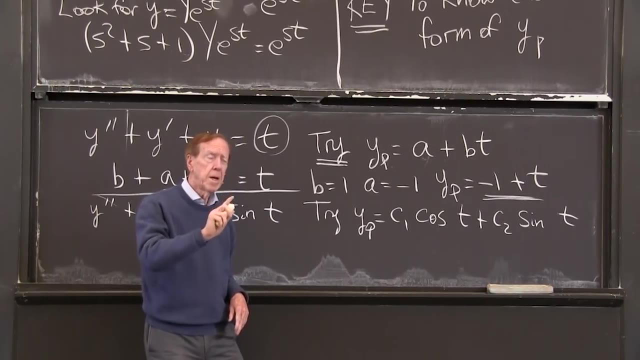 the equation correct by choosing a good sine c1 and c2.. I just noticed that you remember from Euler's great formula that the cosine is a combination of e to the it and e to the minus it. So in a way we're really using the original example. 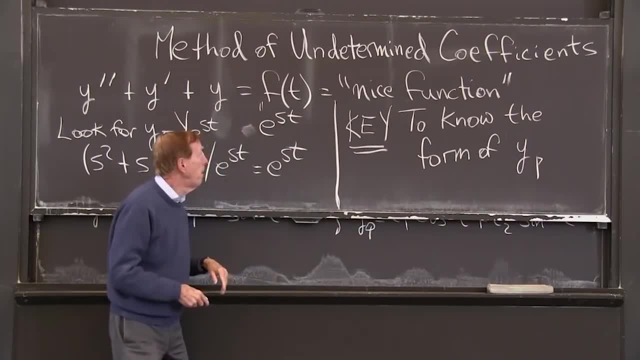 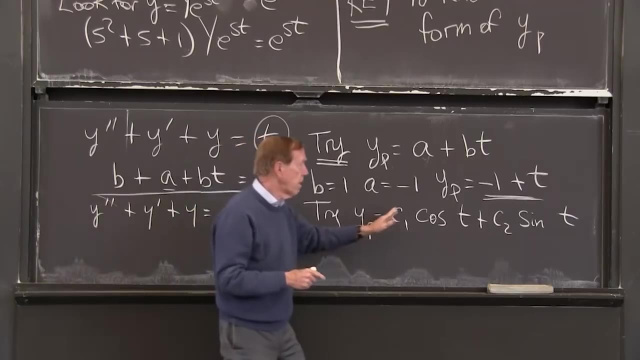 We're using this example- e to the st- with two s's: e to the it And e to the minus it. So we have two exponentials in a cosine. So I'm not surprised that there are two constants to find. 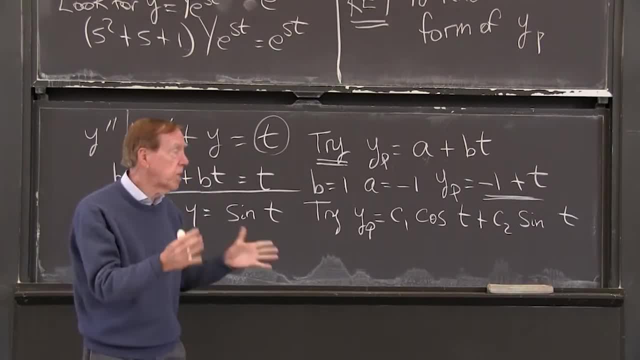 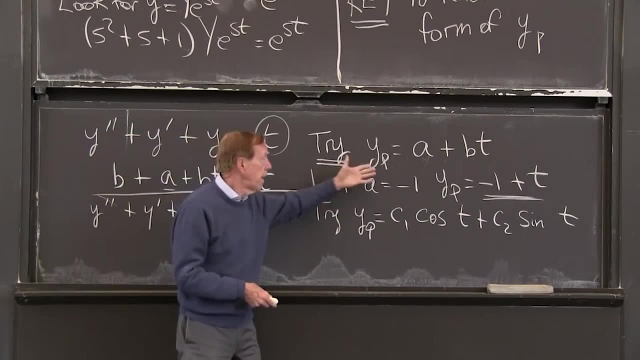 And now, finally, I have to say, is this the end of nice functions? So nice functions include exponentials, polynomials. These are really exponentials, complex exponentials, And then we have a constant. And now there's one more possibility. 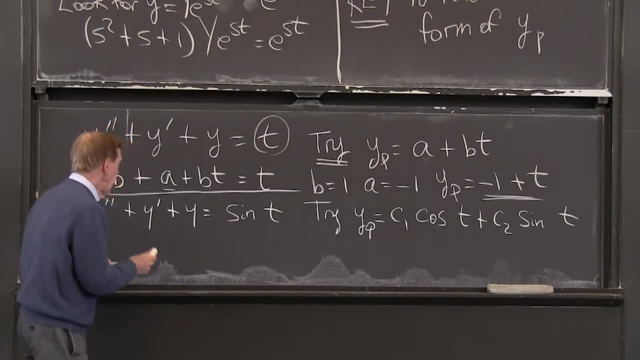 that we can deal with in this simple way, And that possibility is a product of. so now I'll show you what to do. if it was t times sine t, Suppose we have the right-hand side, the f of t, the forcing term is t times sine t. 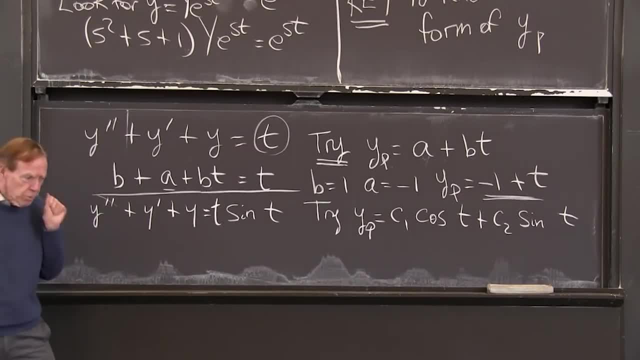 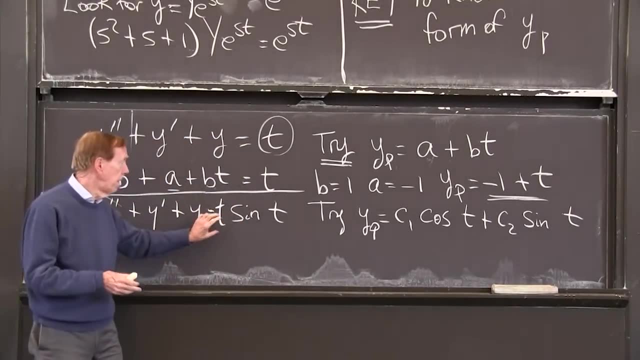 What is the form to assume? That's really easy, That's really. all you have to know is what form to assume. OK, Now that t. so we have here a product, A polynomial times, a sine or cosine or exponential. 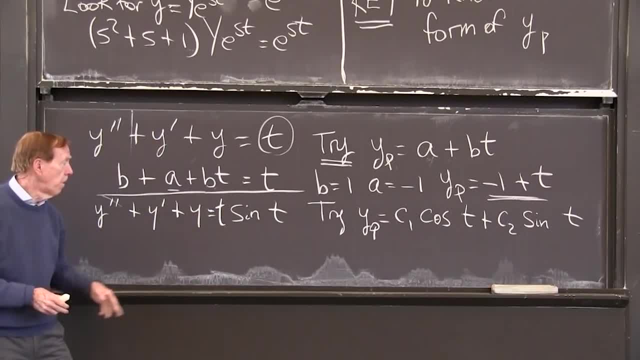 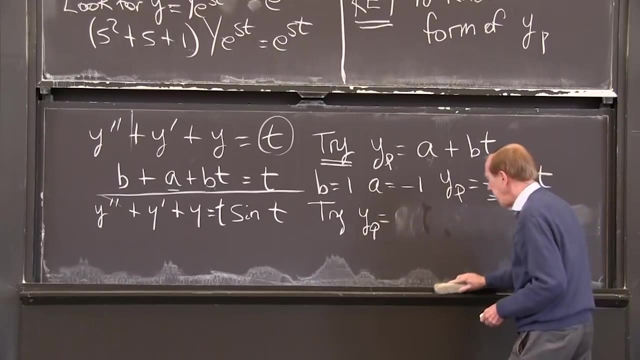 I could have done t e to the st there, So let me. but what do I have to do when the t shows up there? Then I have to try something more with a t And there. so now I have a product of polynomial times sine cosine or exponential. 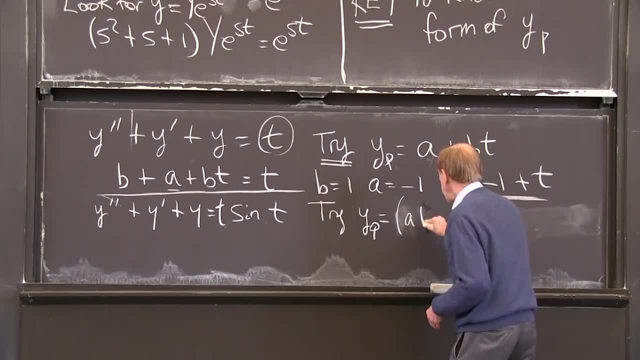 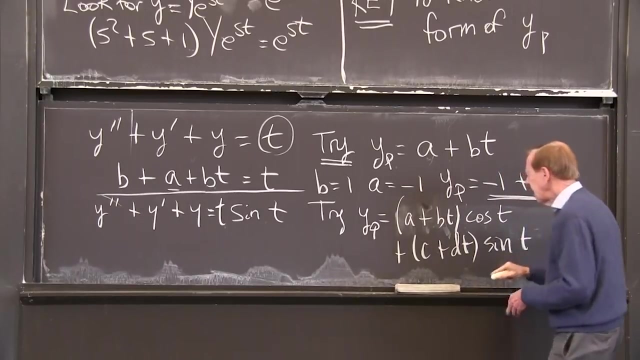 So what I try is a t plus, or rather a plus b t. I try a product times cos t and c plus d t. OK, Times sine t. That's about as bad a case as we're going to see, but it's still quite pleasant. 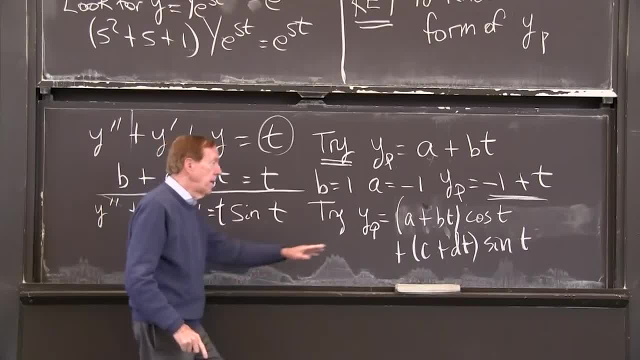 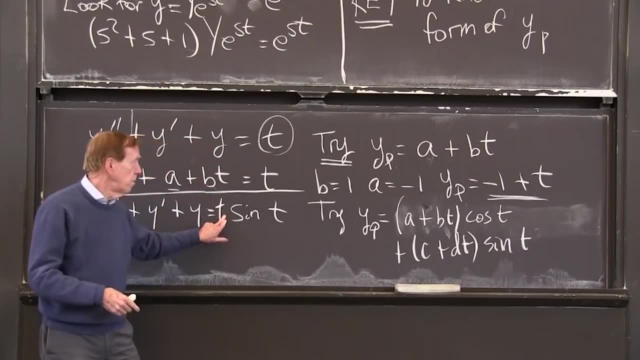 So what do I see there? Because of the t here I needed to assume polynomials up to that same degree, 1.. So a plus b t. I had to do that just the way I did up there when there was a t. 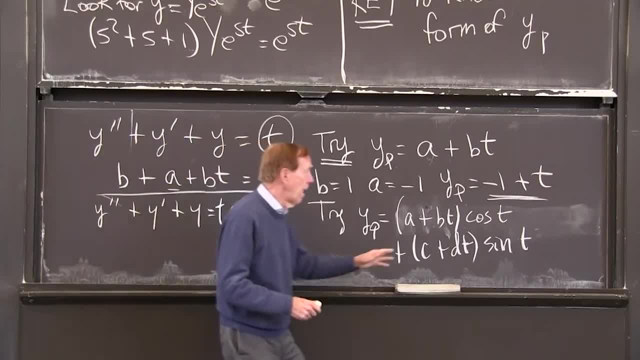 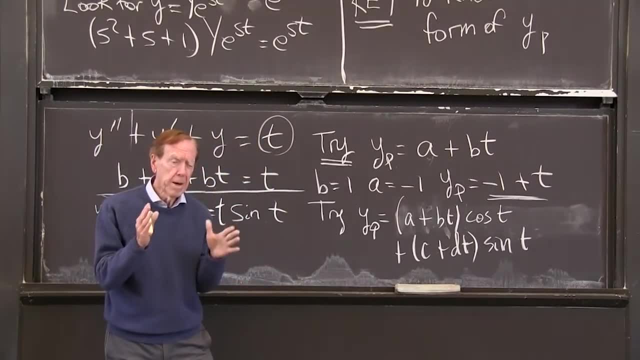 But now it multiplies sine t. So I have to do that, I have to allow sine t and also cosine t. The pattern is really- we've sort of completed the list of nice functions- Exponentials, polynomials and polynomial times. exponential: 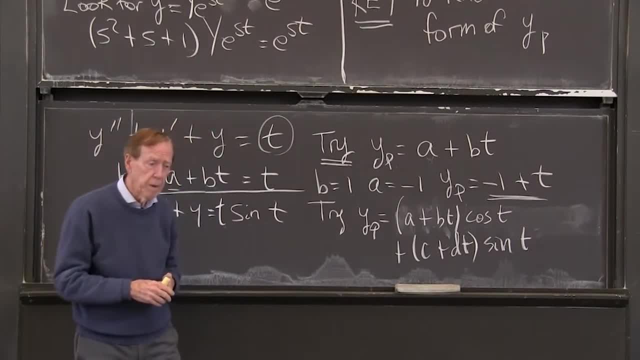 That's really what a nice function is. A polynomial times, an exponential, Or we could have a sum of those guys. We could have two or three polynomial times exponential, Like there, and another one, And that's still a nice function. And what's the real key to nice functions? 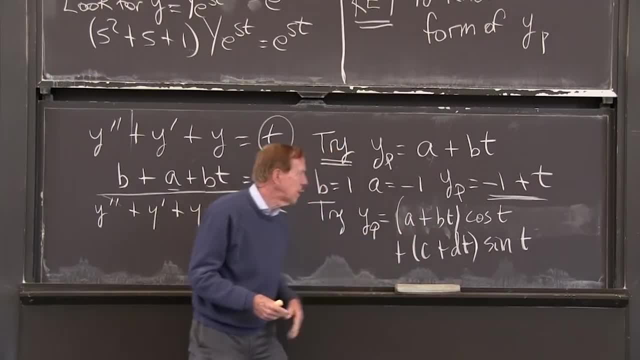 The key point is: why is this such a good bunch of functions? Because if I take its derivative, I get a function of the same form. If I take the derivative of that right-hand side and I use the product rule, you see I'll get this times the derivative. 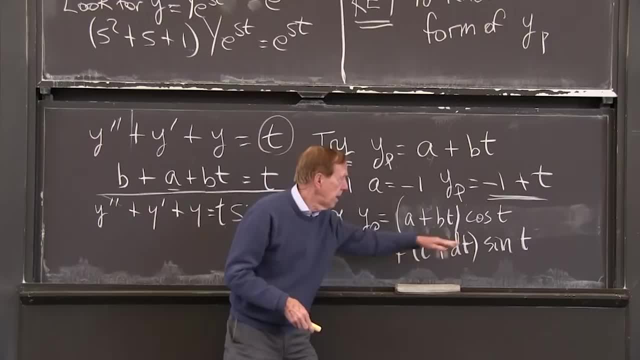 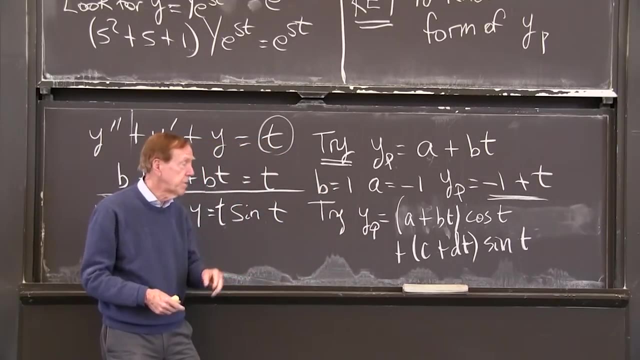 OK, The derivative of that. So I'll have something looking with a sine in there And I get this times the derivative of that which is just a b. So again it fits the same form: Polynomial times cosine. polynomial times sine. 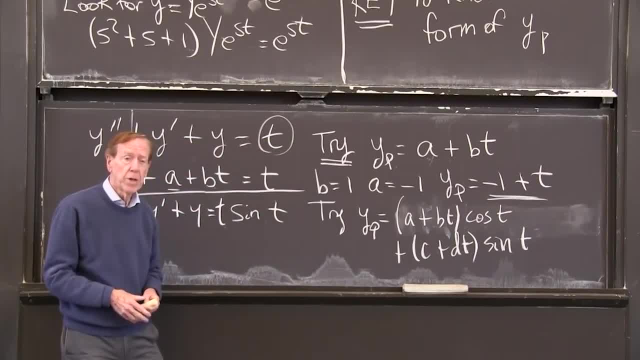 So here I have a case where I have actually four coefficients, But they'll all fall out. when you plug that into the equation, You just match terms And you're golden. So it really is a straightforward method, Straightforward. And so the key about nice functions is: 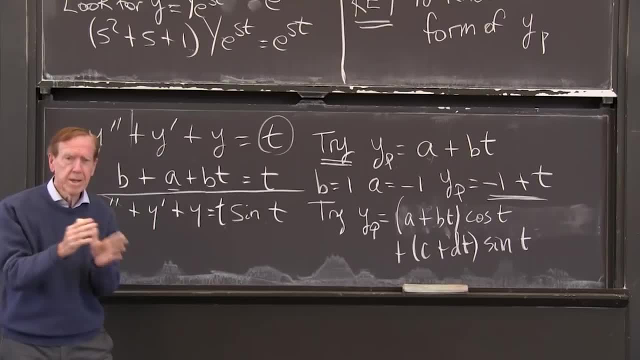 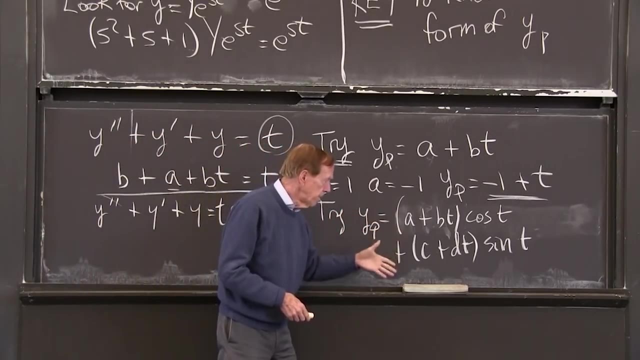 and they're nice for Laplace transforms. They're nice at every step. It's the same good functions that we keep discovering as our best examples. The key about nice functions is that that's a form of a nice function, because its derivative has the same form. 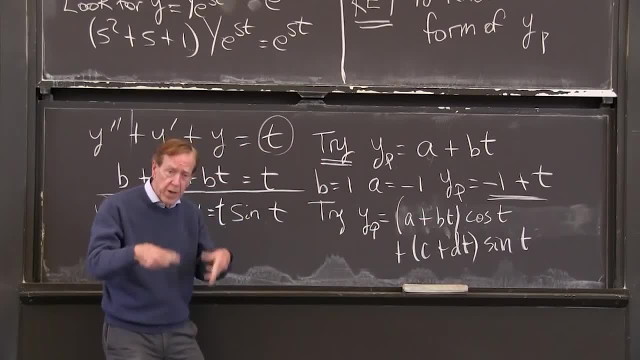 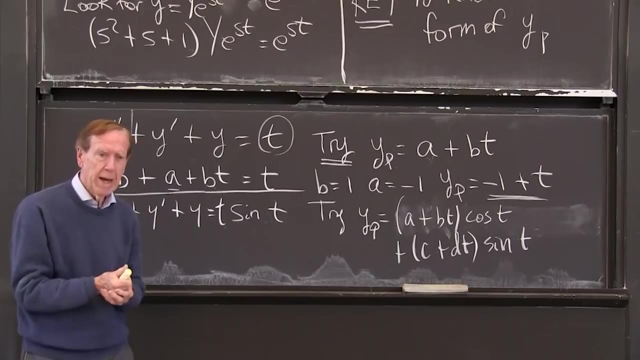 The derivative of that function fits that pattern again, And then the second derivative fits, All the derivatives fit. So when we put them in the equation, everything fits. And always in the last minute of a lecture there's a special case. There's a special case. 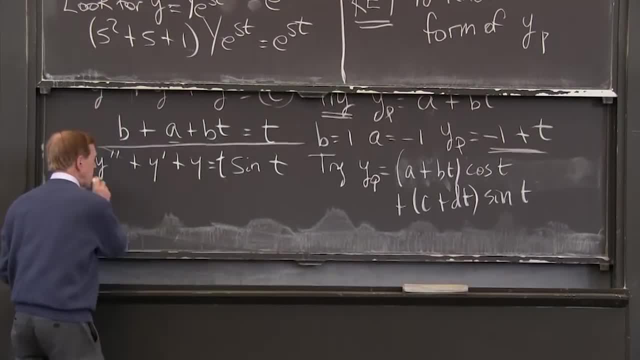 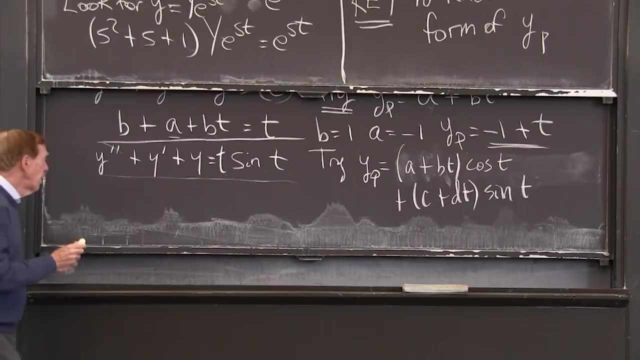 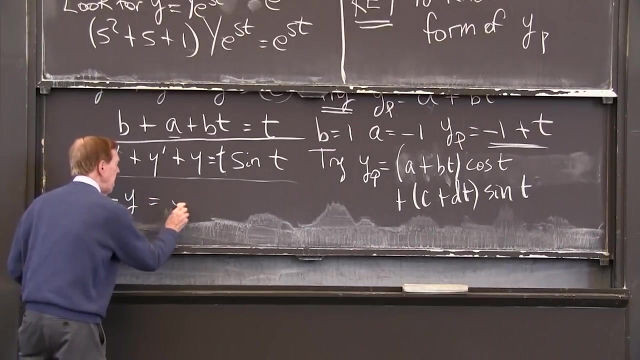 And let's remember what that is So special case. when we have to change the form, And why would we have to do that? Let me do y double prime minus. y, say is e to the t. What is special about that? 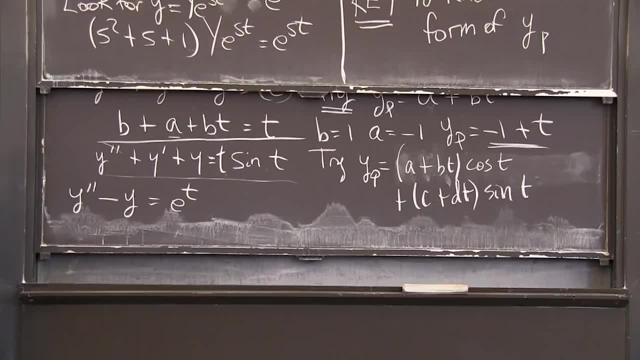 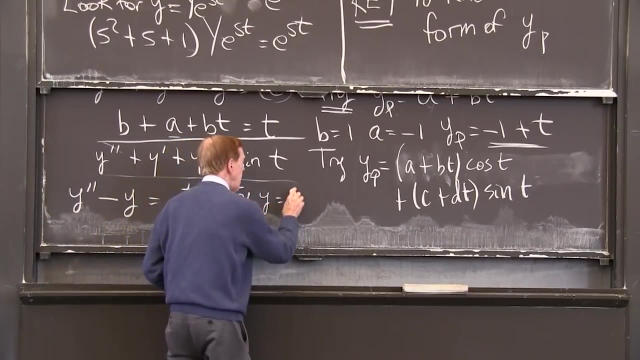 What's special is that this right hand side, this f function, solves The equation. If I tried to assume. if I try e to the t it will fail. Try y equals some y e to the t. Do you see how that's going to fail? 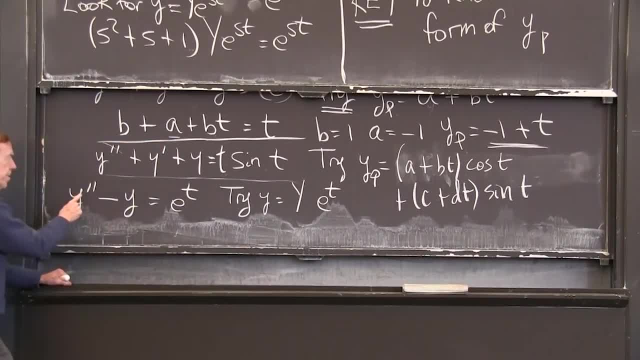 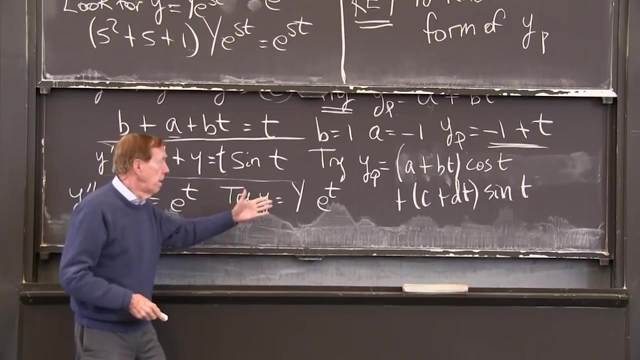 If I put that into the equation, the second derivative will cancel the y and I'm 0 on the left side. Failure, Because that's the case called regression, Right Resonance. This is a case of resonance When the form of the right hand side. 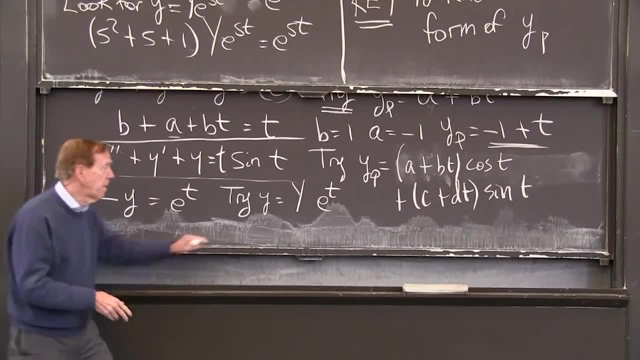 is a null solution. at the same time, It can't be a particular solution. It won't work because it's also a null solution. And do you remember how to escape resonance, How to deal with resonance? What happens with resonance? The solution is a little more complicated. 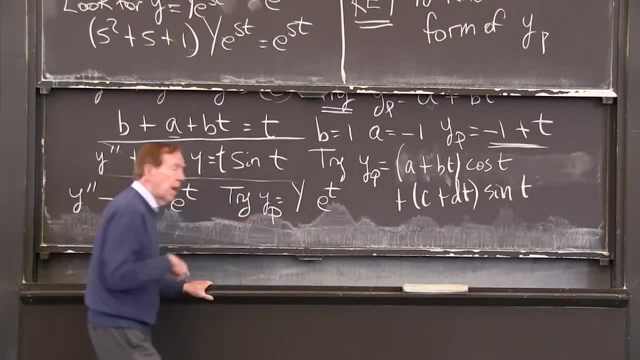 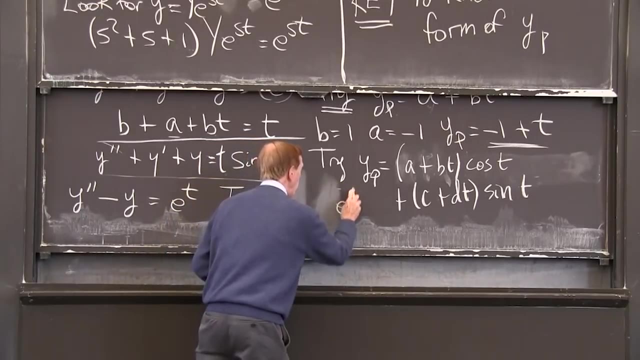 but it fits everything here. We have to assume to allow a t. We have to allow a t. So instead of this multiple of e and in this thing we have to allow, So I'm going to assume I have to have, I need a t in there. 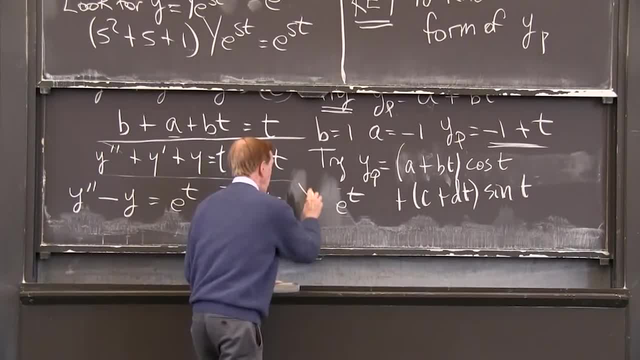 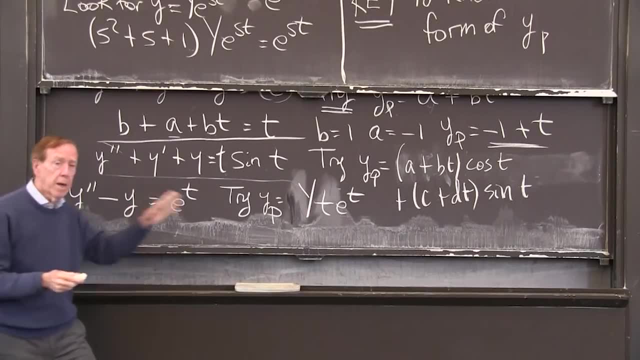 Oh no, actually I don't know, I just need a t That would do it. That would do it When there's resonance t, Take the form you would normally assume and multiply by that extra factor t. Then, when I substitute that into the differential equation, 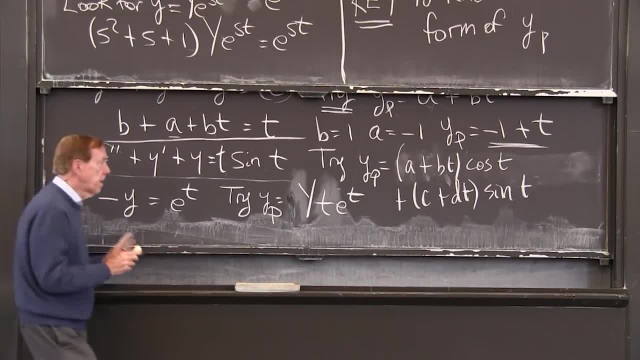 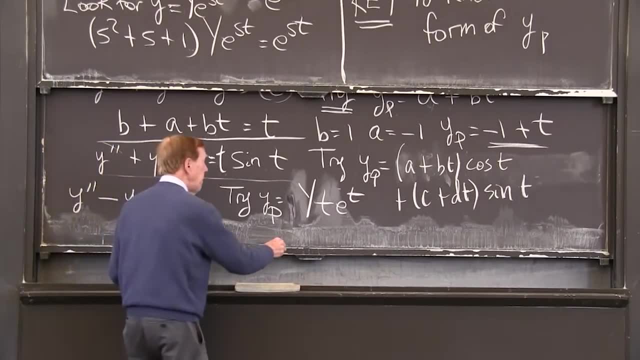 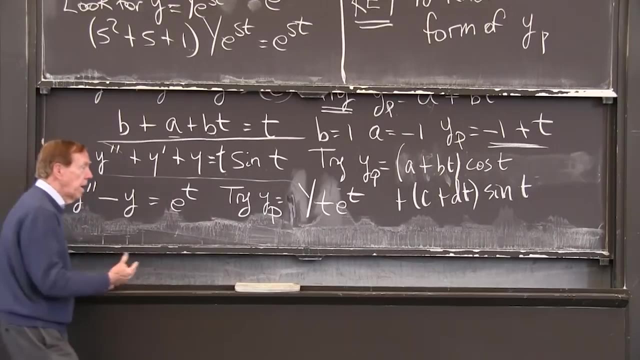 I'll find y quite safely. I'll find y entirely safely, Shall I do that. So that's the resonant case, The sort of special situation when e to the t solved this. So we need something new and the way we get the right new thing is to have a t in there. 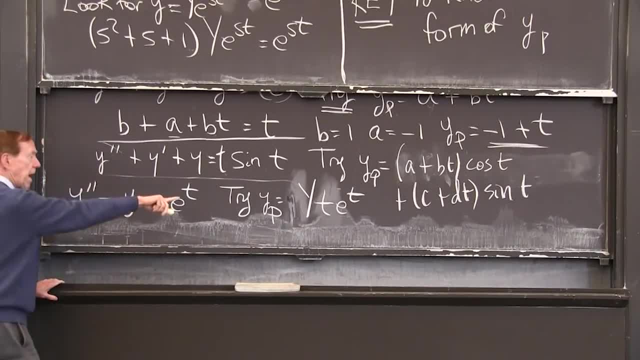 So when I plug that in, I take the second derivative of that subtract off that itself. match e to the t and that will tell me the number y. Perhaps it's 1, half or 1.. I won't do it. 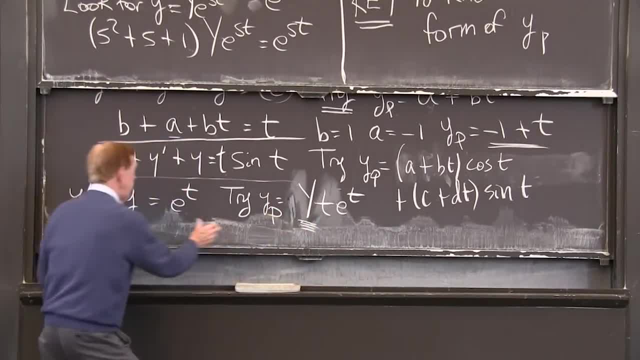 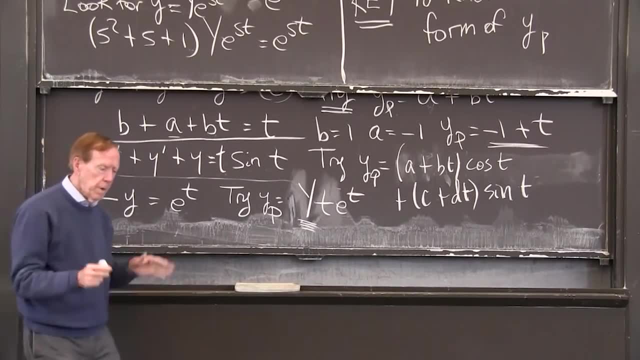 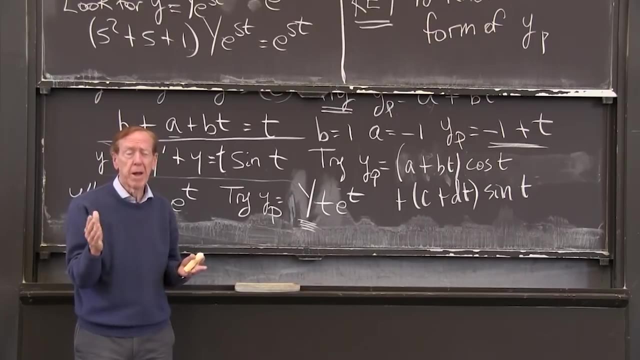 Maybe I leave that as an exercise, Put that into the equation and determine the t Number, capital, Y. OK, Let me pull it together. So we have certain nice functions which we're going to see again because they're nice. Every method works well for these functions. 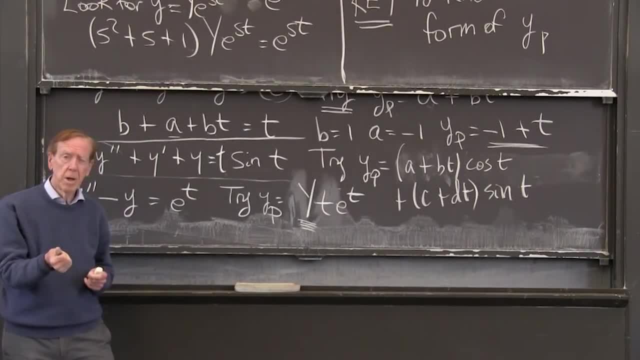 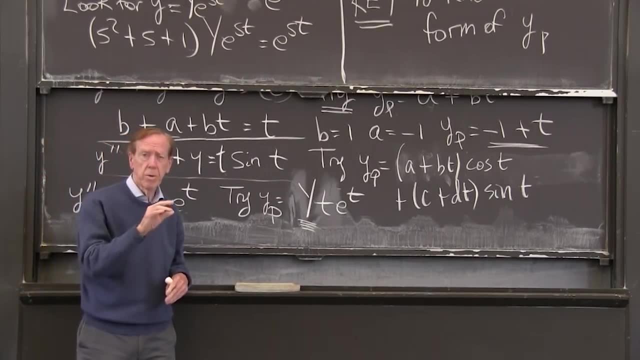 And these functions are exponentials, polynomials or polynomials, times exponentials, And within exponentials I include sine and cosine. And for those functions we know the form, We plug it into the equation, We make it match, We choose these undetermined coefficients.